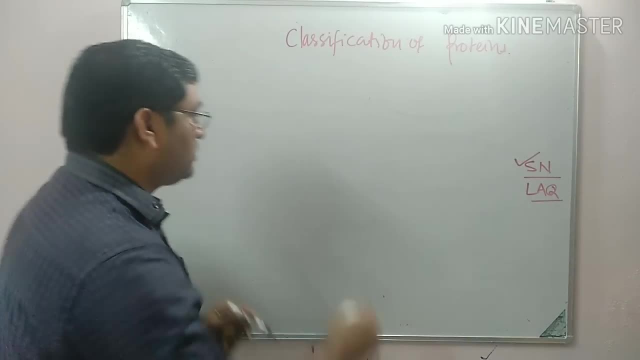 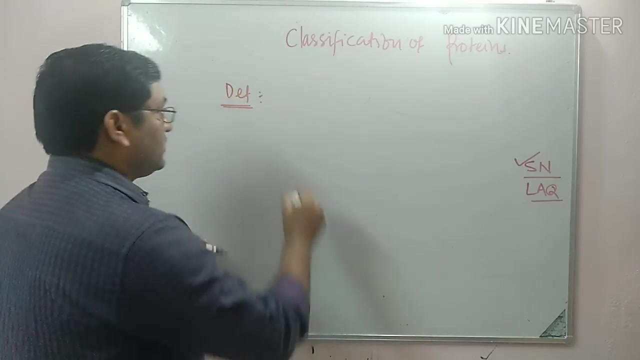 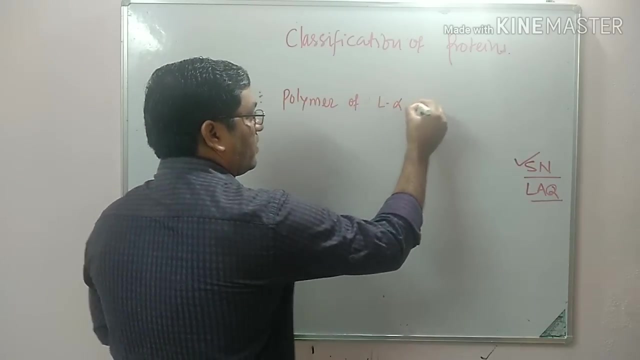 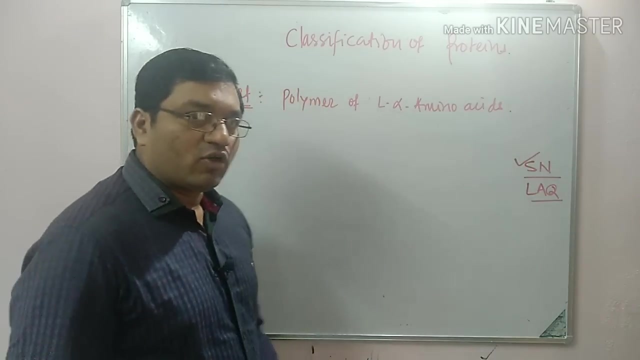 So, coming to the discussion of proteins, First we will discuss the definition in short, or definition These proteins. they are polymer, Polymer of L alpha amino acids, Amino Acids. So proteins are polymer of amino acids, They are polymer of L alpha amino acids. Okay, 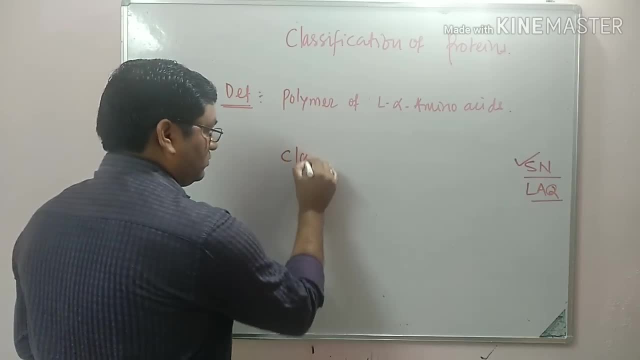 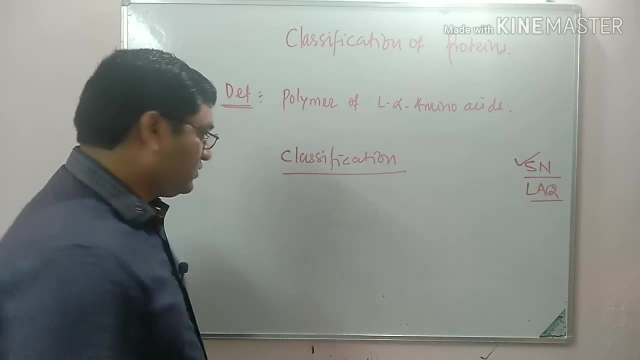 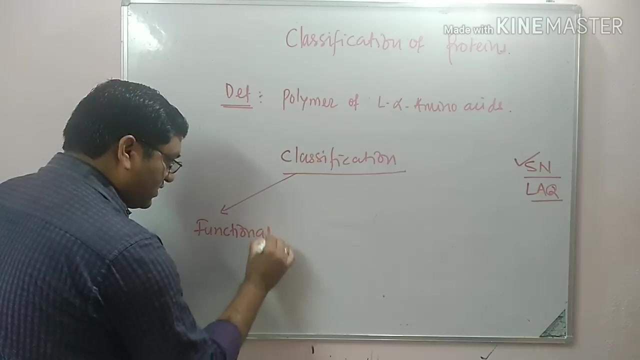 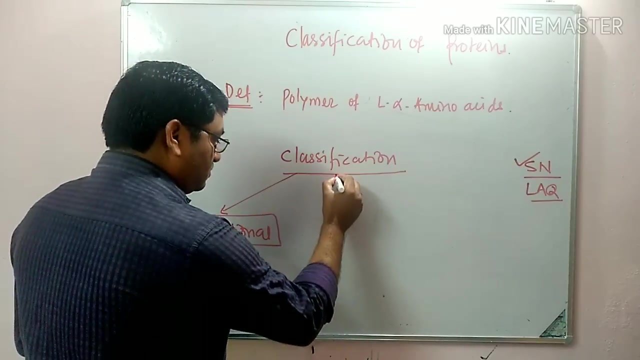 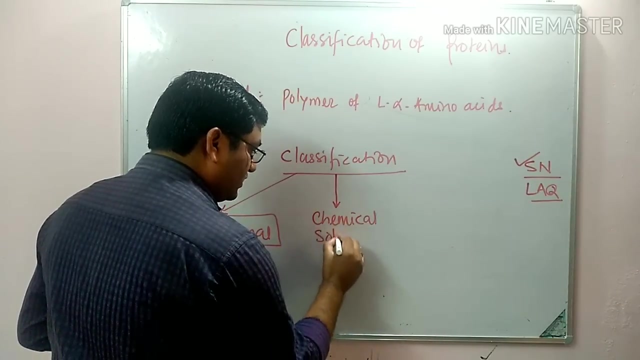 Now coming to the classification Classification Protein. they are classified on the basis of their functions. First, the functional classification, And it is a very, very important short note In university exam. Second is the based on their chemical nature, Chemical nature and solubility. 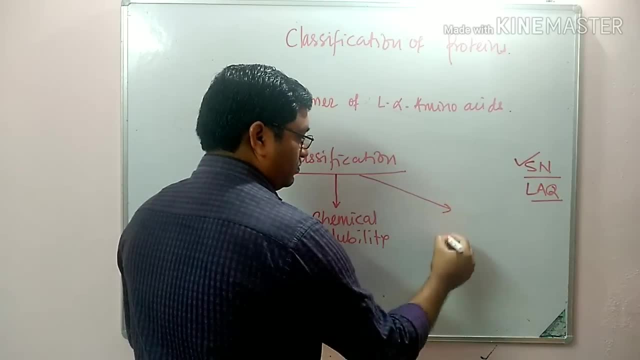 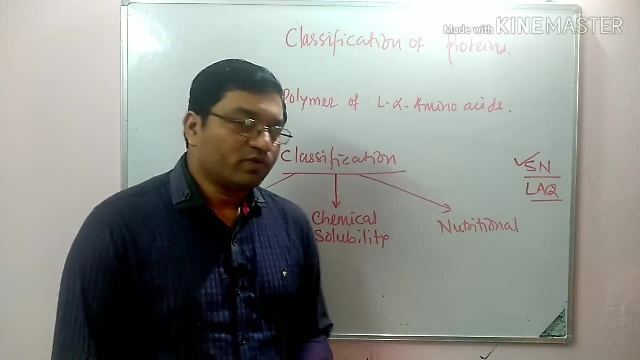 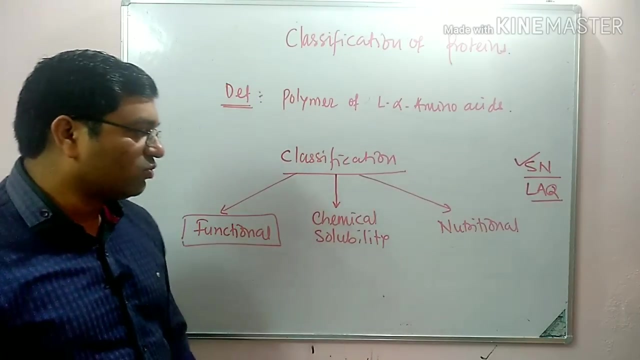 And third one is the based on their nutritional status: Nutritional classification. So these are the three basis on which proteins they are classified or proteins are classified: Functional classification based on chemical nature and solubility, And nutritional classification based on classification. On the basis of first, we will discuss the functional classification, And this is a very Great 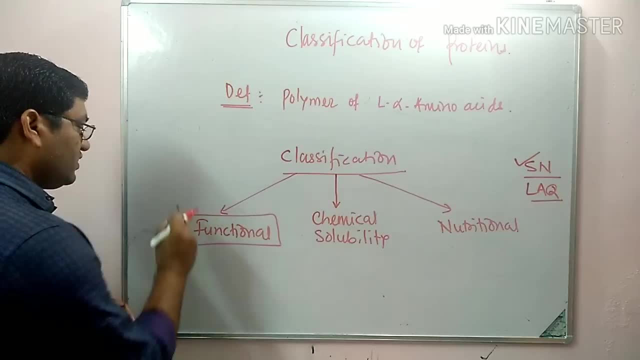 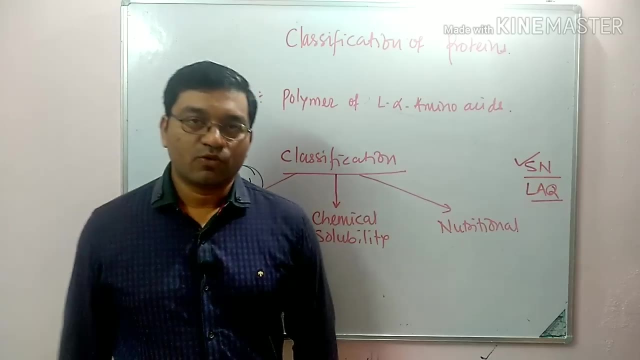 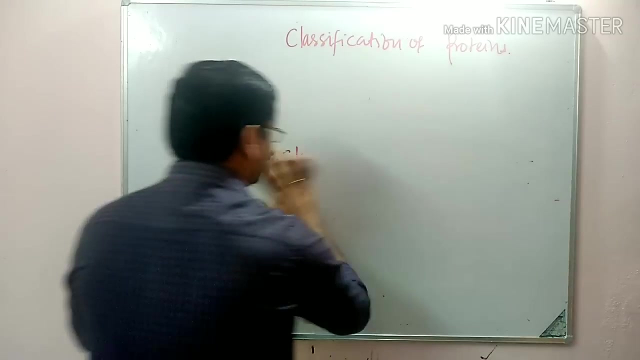 On the basis of. first, We will talk about the functional classification, And this is a very Important Short note in university examination: Functional classification ofes. Okay, Now coming to the functional classification of proteins. Functional classification of kilometer protean. 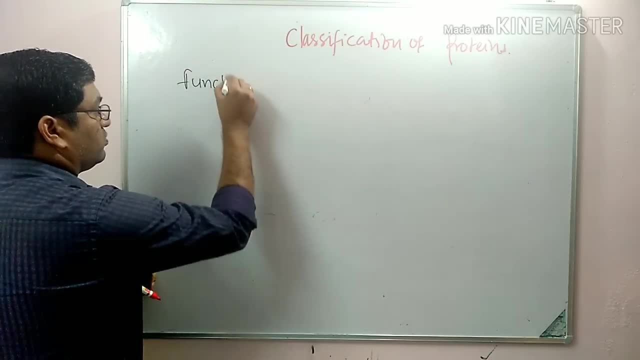 Okay, So protein, their vital動画. they are from the same age as thecoins, So these are already Americans that are from the age of 10 years. Okay, Now let us discuss the function classification of proteins, at the same as the while crítiques for protein. So let us look at the. These are the two ingredients, And they are anything and not anything. That means protein, That is thatact leicht itchwege anymore Physically, And then we will discuss fundamental classification of proteins, So that today I have I told that�� apart. multiple of these four local luxury carriers are agony. 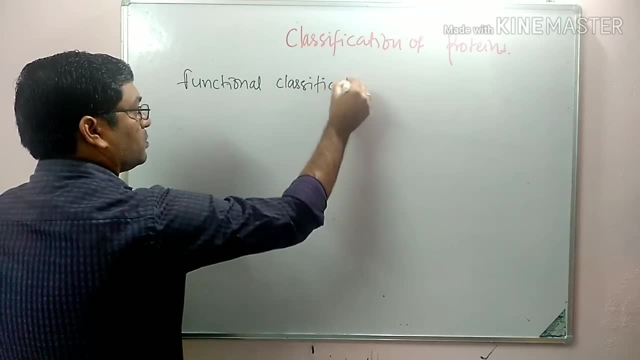 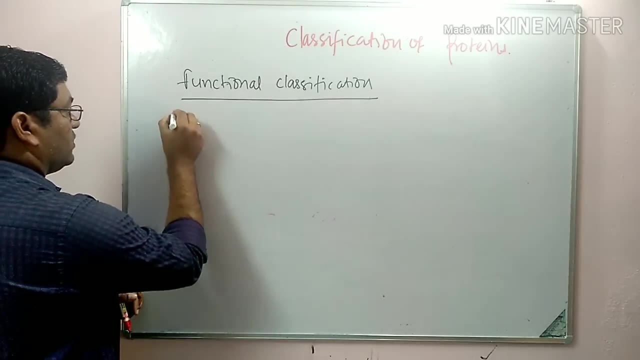 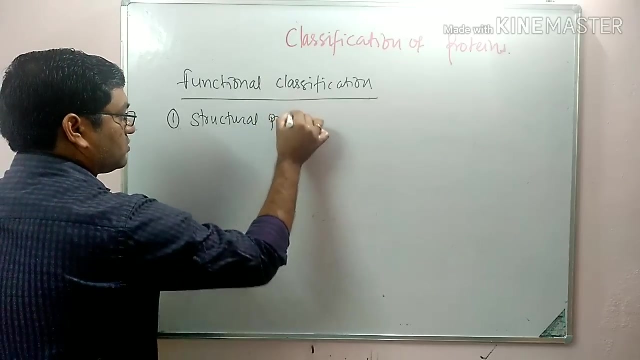 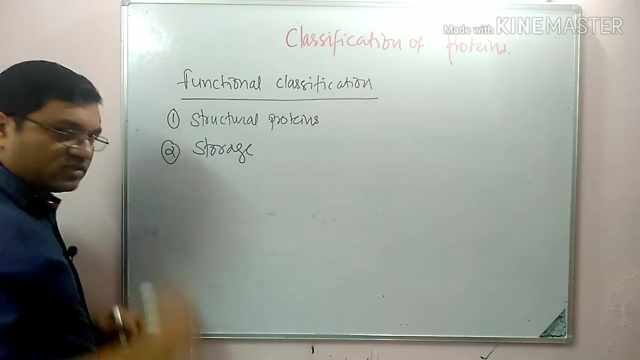 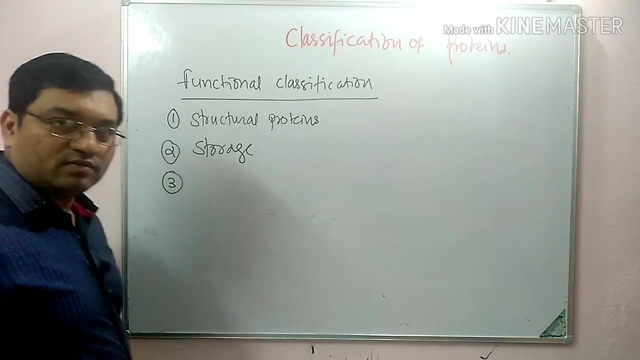 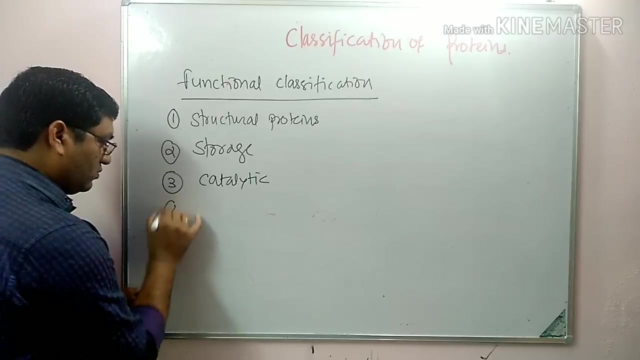 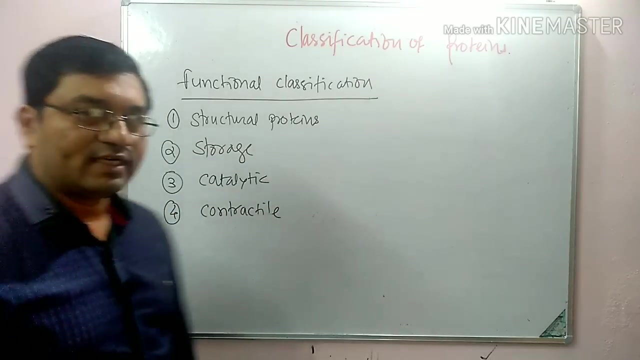 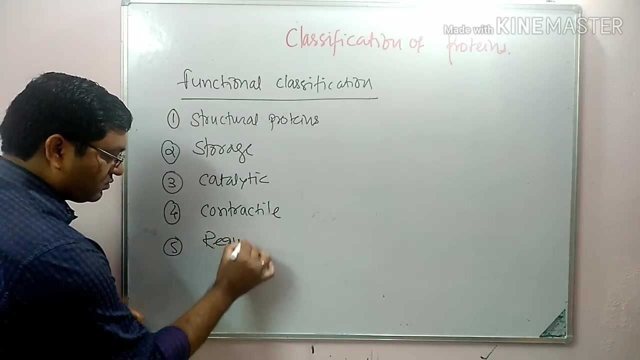 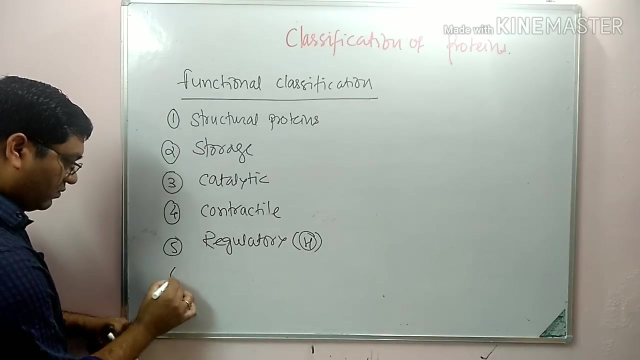 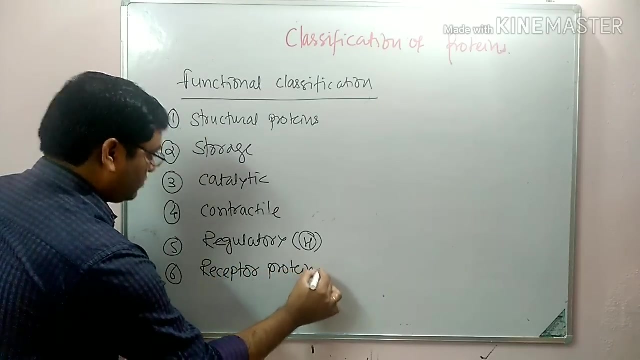 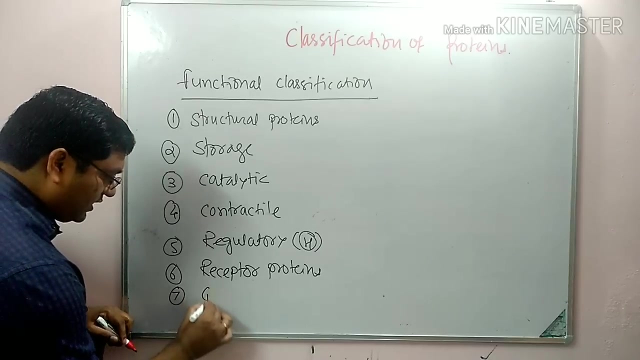 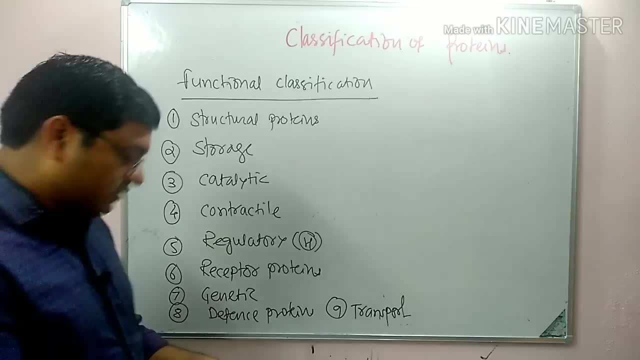 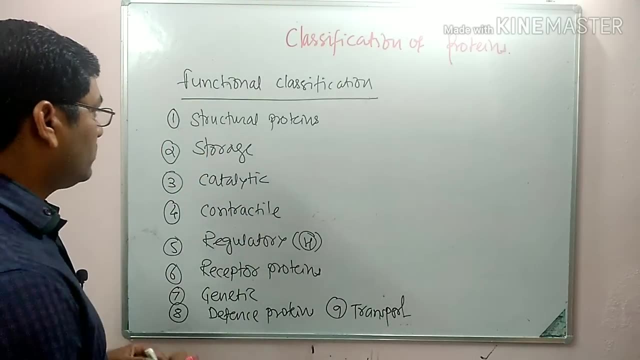 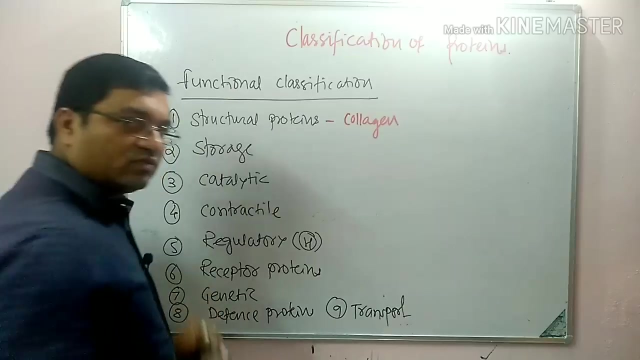 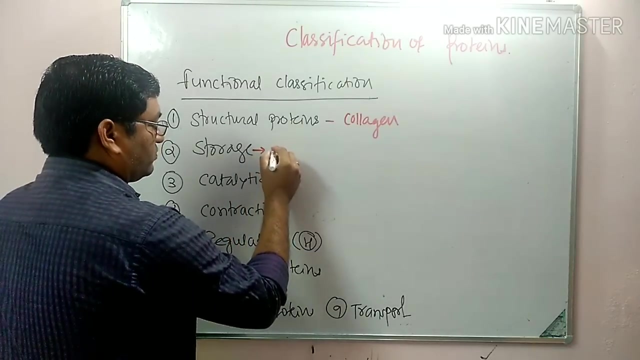 SC them animal. these are the classification of proteins u all beings, all the personal products and food, on the basis of just function. now, coming to the example: structural protein Smith: they are responsible for structure. okay, it includes bridges. it includes bridges. now, coming to the example: structural protein Smith: they are responsible for structure. okay, it includes privileged. 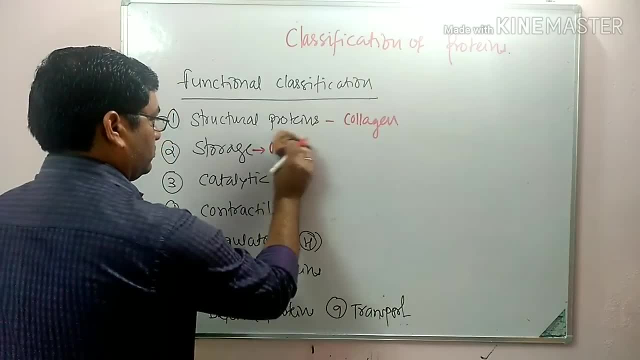 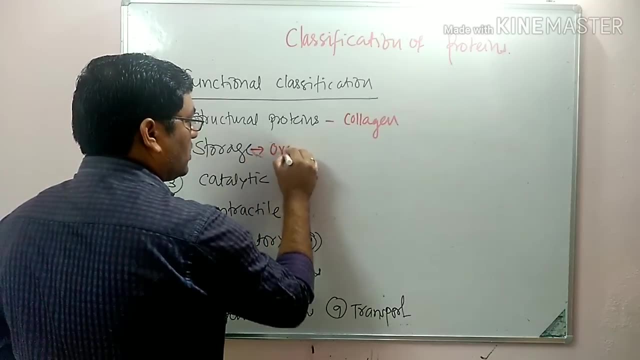 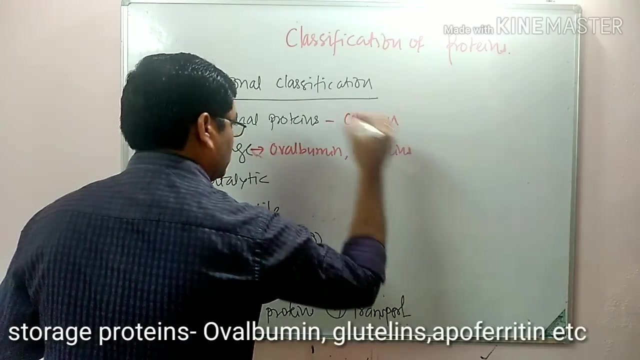 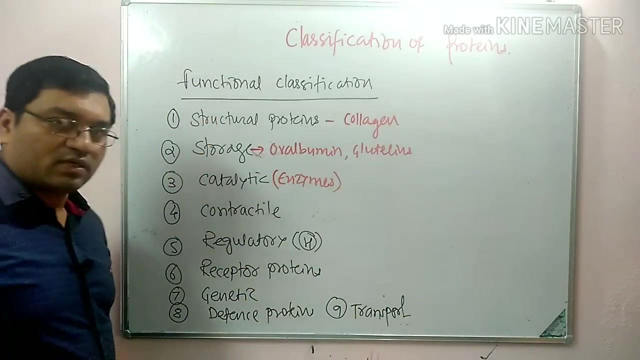 collagen, collagen. What is a structural protein? okay, then wanted to carry away哈囉 albuming Bunny 해 In storage protein. it includes Ovalbumin, Glutalins, Etc. Catalytic means enzymes. Okay, Enzymes. Write down the name of enzymes. 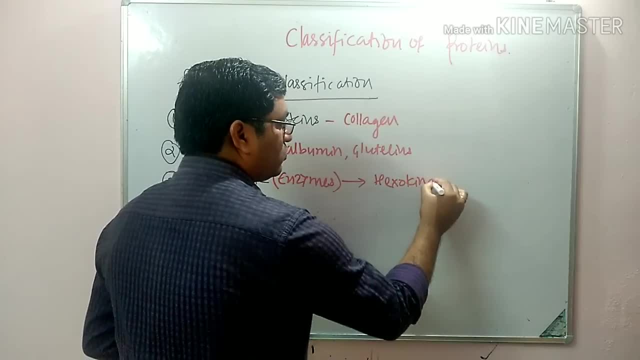 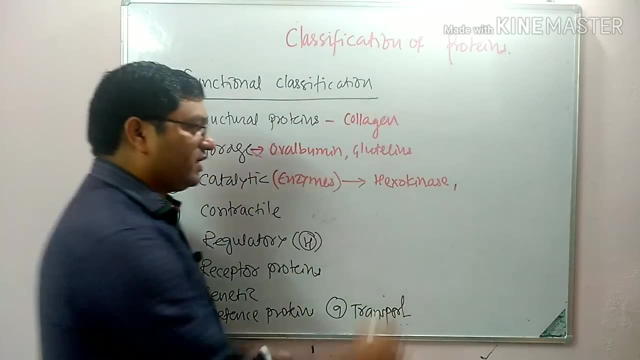 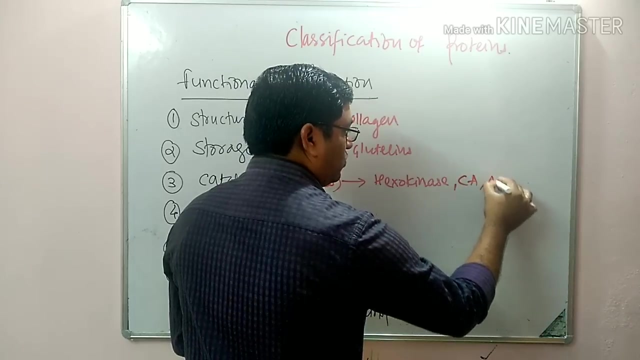 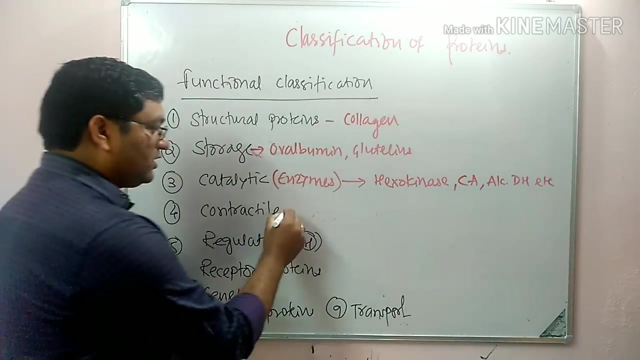 Example: Hexokinase, Glucokinase, Etc. Carbonic anhydrase. Write down Hexokinase, Carbonic anhydrase, Alcohol, dehydrogenase, Etc. Okay, Then contractile protein. They are responsible for muscle contraction. Actin. 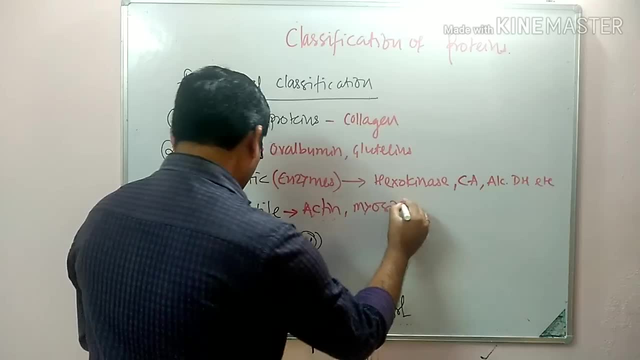 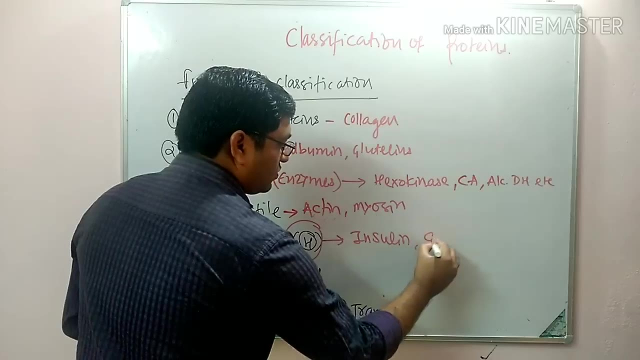 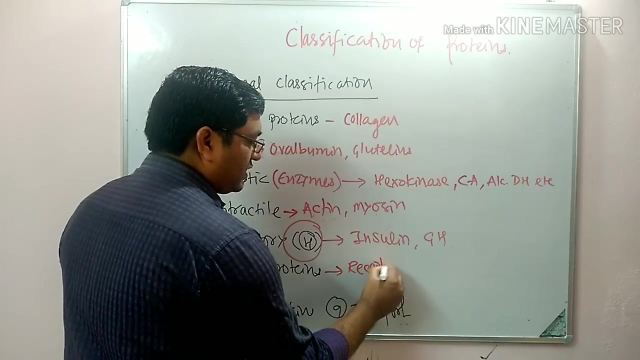 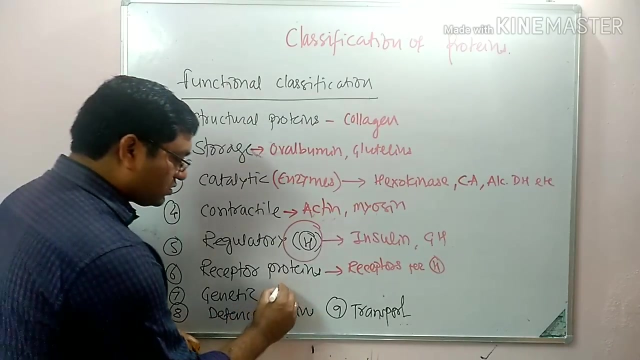 Myosin. Regulatory protein means Hormones. It includes Insulin, Insulin, Growth hormone. Okay, Etc. Receptor proteins. they act as a receptor, They act as a receptors for hormones. Okay Then genetic protein. it includes Nucleoprotein. 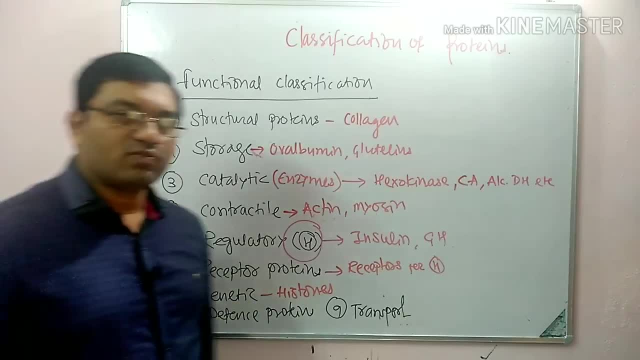 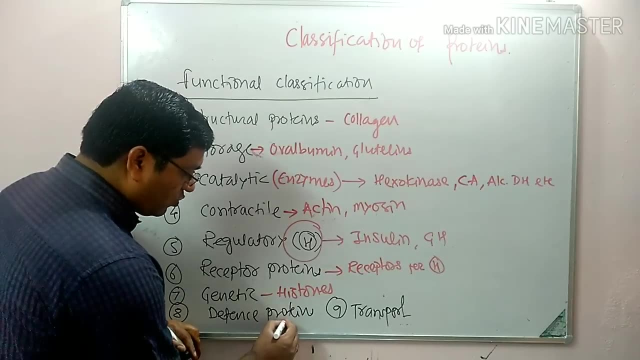 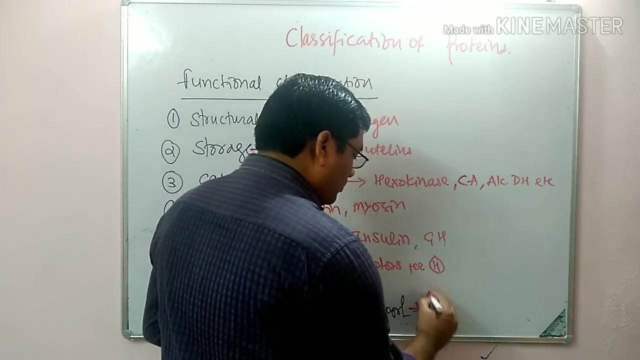 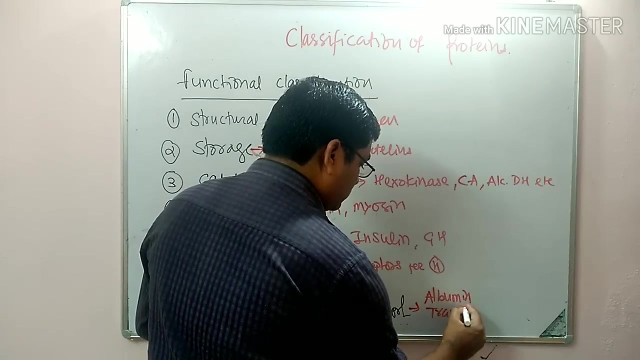 That is, histones. Histones, they are basic proteins. They are found in association with nucleic acid, Genetic proteins. Then defense protein: It includes immunoglobulins, Immunoglobulins, Immunoglobulins And transport protein. it includes albumin, transferrin, celluloplasmin, etc. 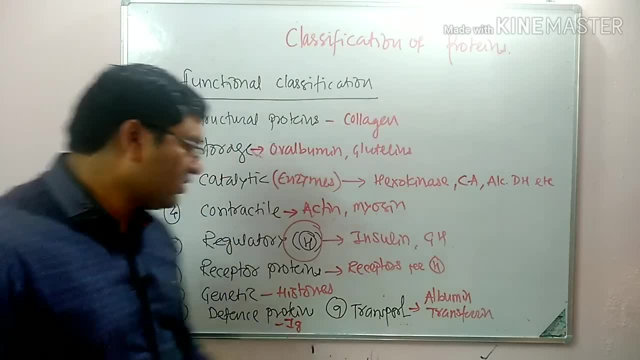 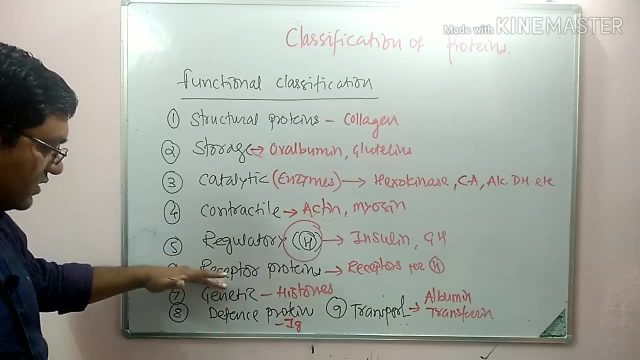 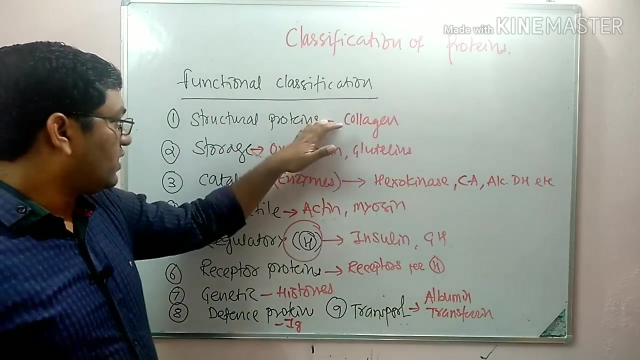 Okay, They are transport proteins. Okay, So this is a functional classification of protein: structural storage, catalytic, contractile, regulatory storage, Regulatory receptor, genetic defense and transport protein. Remember one-one example of each Structural protein: collagen storage protein, glutinous ovalbumin, catalytic enzyme. 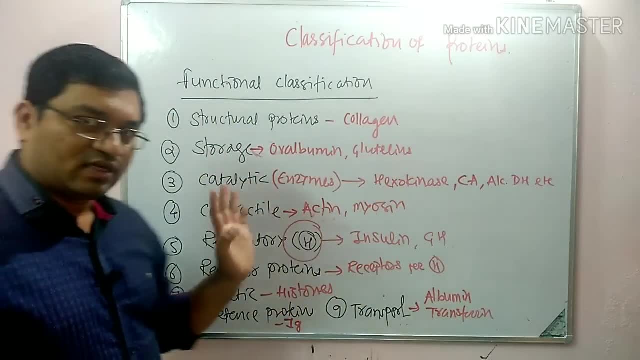 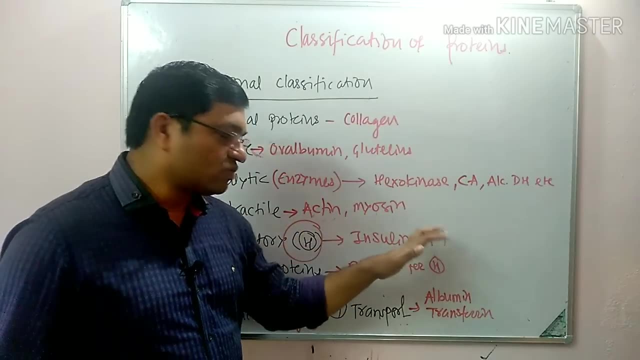 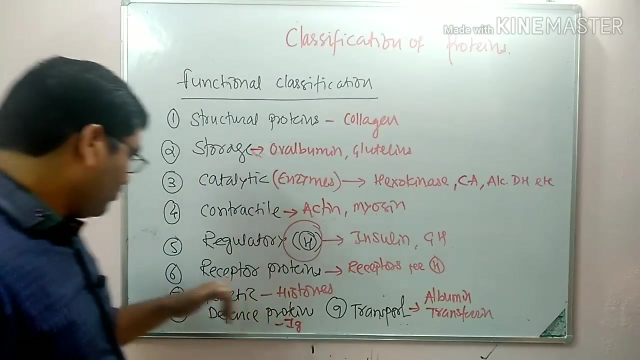 Write any name of any enzymes except RNA, Contractile actin and myosin, Regulatory protein hormones, insulin growth hormone. Write down the name of peptide hormones only Not steroid hormones. Okay, Then receptor proteins: they act as a receptors. 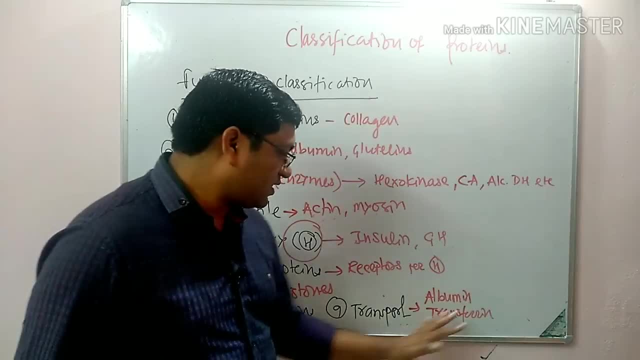 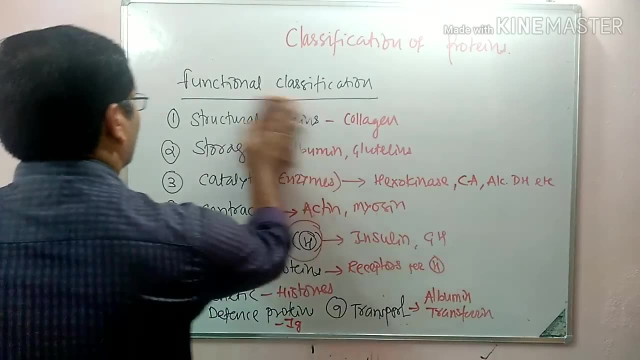 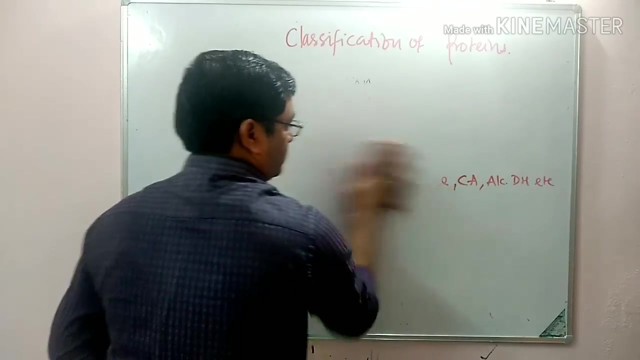 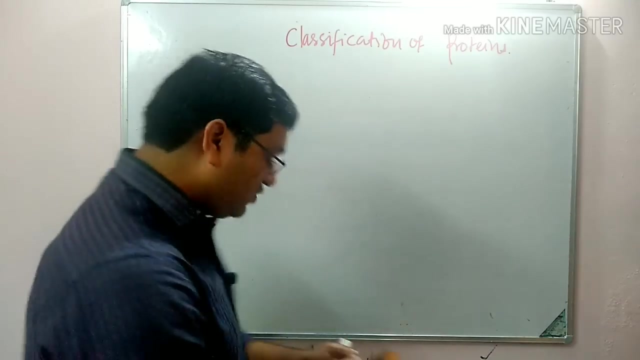 Then genetic protein, histones, defense protein, immunoglobulin and transport protein albumin. So this is a functional classification of protein. Now moving to the classification of protein based on their chemical nature and solubility. Functional classification is very, very important and frequently asked questions in university. 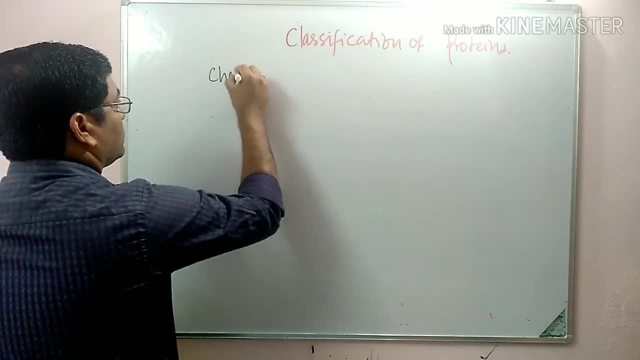 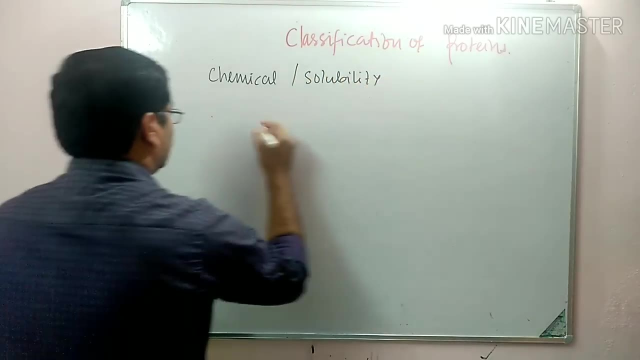 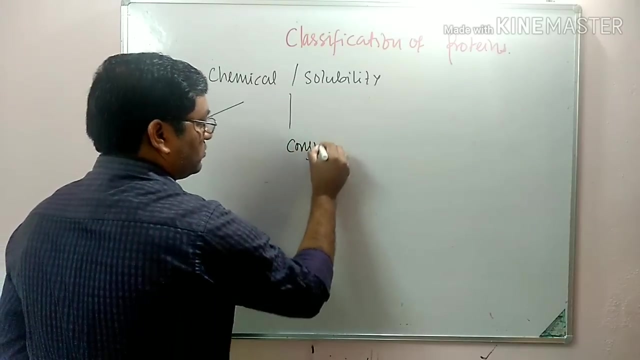 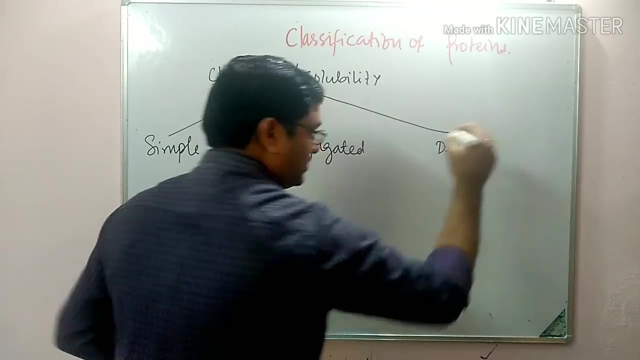 exam. Then, based on their chemical nature and solubility, they are simple proteins, then conjugated and derived. It is very simple. It is similar to that of lipid classification. Simple proteins means they are composed of amino acids, So it is very simple. There are no amino acids, only amino acids. no prosthetic group is there. In conjugated protein, there is amino acid plus prosthetic group or additional group is there? apart from this, amino acids and derived means: they are derived from this simple and conjugated proteins. 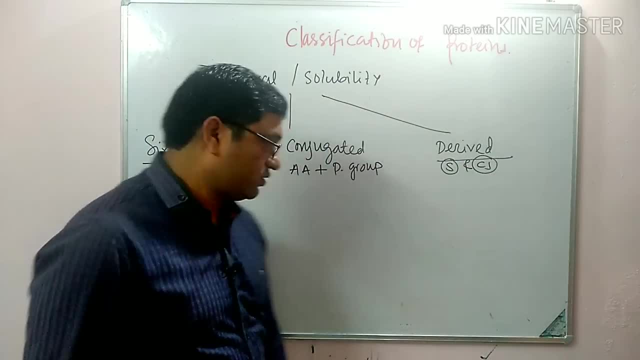 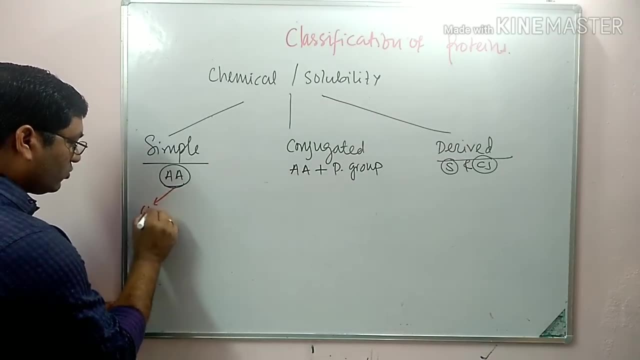 They are derived from simple and conjugated protein. In simple protein it is again classified into amino acids, So it is very simple. So you think we are some people who are simple anddroids, What they are meant to be. If they are not, then you can define them as NaP protein, Mp1 protein, CrInP protein, ClP protein. 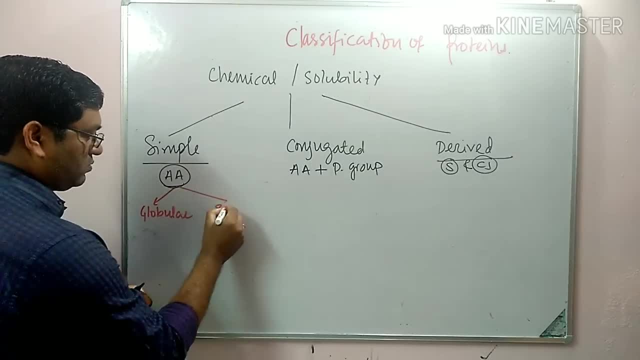 Re-CJ protein. We are not just unaware of NaP. it is that same thing BY each one. they are different, So let us say they areunchified. Say that two times to 야 is equal to one, So let us just sum up. 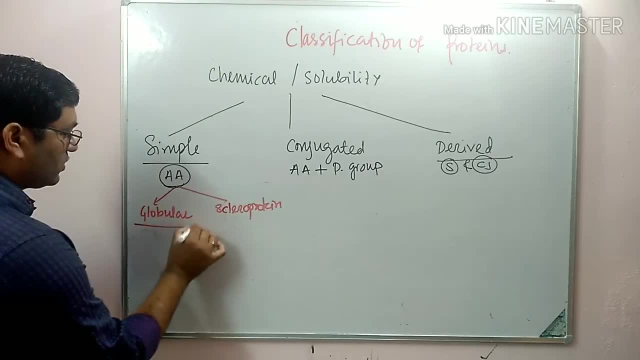 So in this case, 1 and the이어, we are not sure of the Mat. They are można우�workeran alpha boardon Supp��. we are missing in the household of definition chopped fe because we are finishing class of lower names or nonreallowed limits. 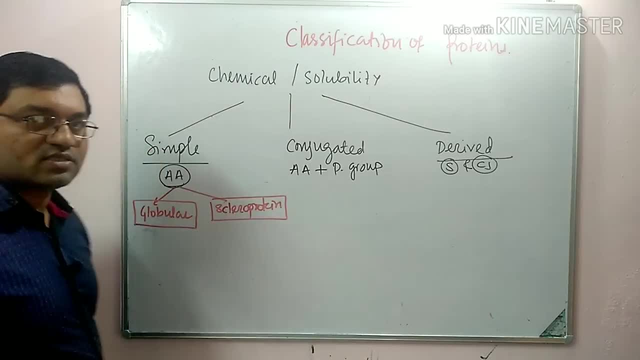 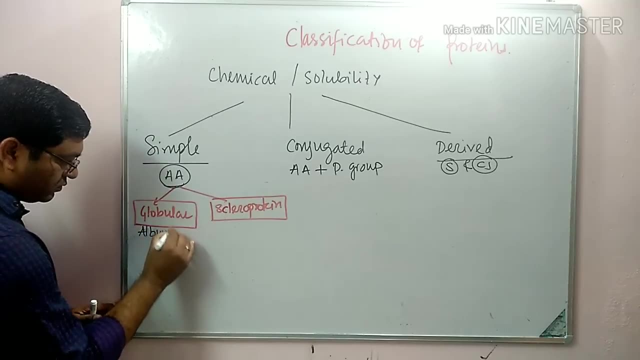 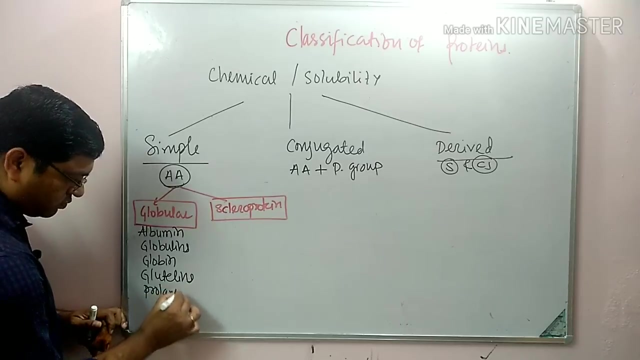 What you can see here is: while污å±o" Stoch smooth домаеä Mirror 8-lガ es bei Then Globulins, Globins, Glutalins, Prolamins, Protamins, Histones. 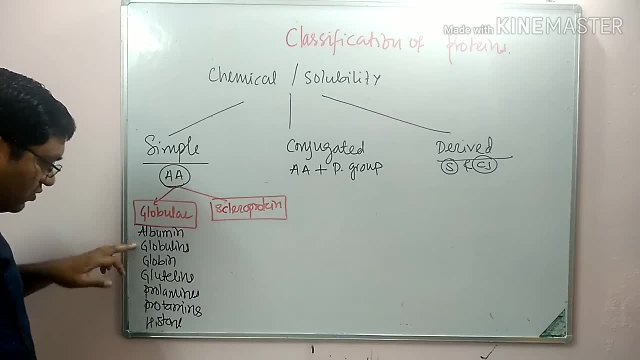 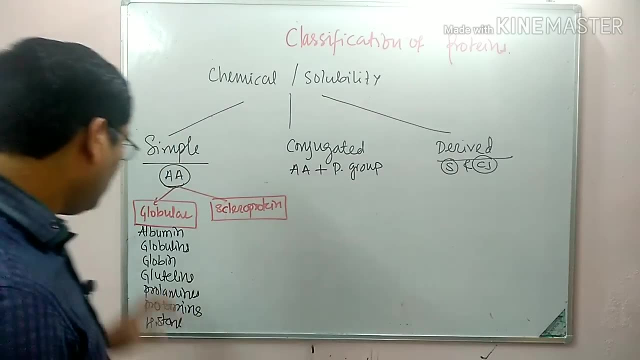 Remember this: Globulins, Albumin, G, G, G, Globulin Globins, Glutalins, P, P, Prolamins, Protamins and Histones. These are the globular proteins. Albumin- Egg Albumin- is the example. 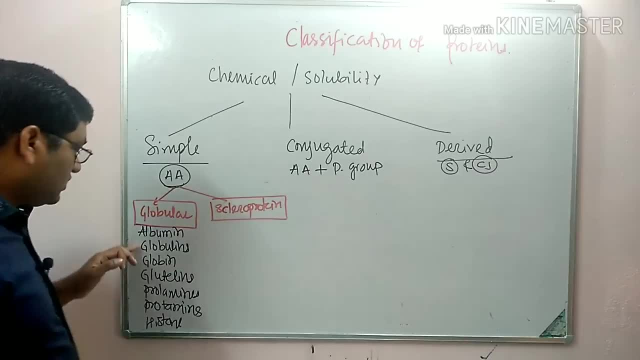 Serum Albumin is the example. Globulins, Serum Globulins. they are example of Globulins: Alpha-1, Alpha-2, Beta Gamma Globulins. Globins are there, Then Glutalins. it is also a storage protein. 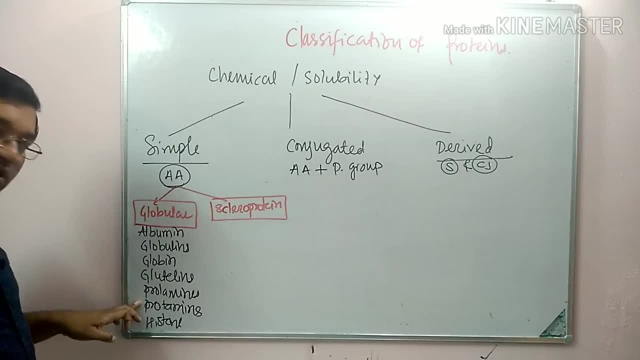 Prolamins and Protamins. Okay, These Protamins, they are found in association with Nucleic Acid. Also, Histone proteins: they are found in association with Nucleic Acids. So these are the globular proteins Soluble in water. Spherical or oval in shape, Then Scleroproteins. it includes Collagen. It is a triple helix Mainly composed of Glycine. Glycine is the major amino acid in Collagen. This is a MCQ. It is a triple helix. Mainly consists of Glycine, Hydroxylysine, Proline, Hydroxyproline and Glycine. Glycine is a major amino acid in Collagen, Then Collagen, Elastine, Elastine. it is found in Tendons, Arteries and Keratin. Keratin. it is found in Skin and Hair. It is found in Skin and Hair, Elastine, Tendons, Arteries Collagen: It is a structural component. It is found in Connective Tissue Collagen. 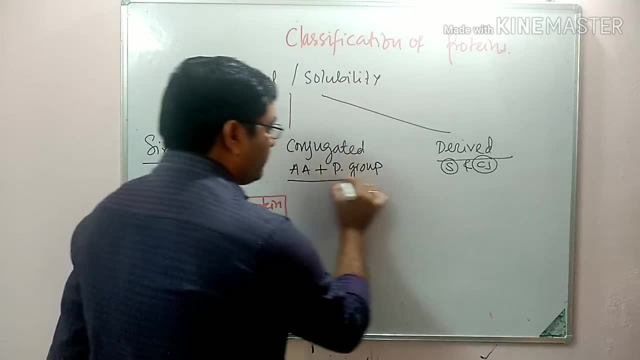 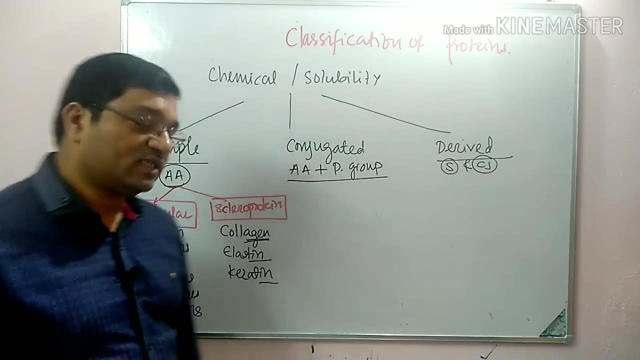 So these are Scleroproteins, Now Conjugated Protein. it is very, very easy to remember. So your chapter starts from the Carbohydrate, then Protein, then Liquid Nucleic Acid. So when it is associated with Carbohydrate, it is known as Glycoprotein. 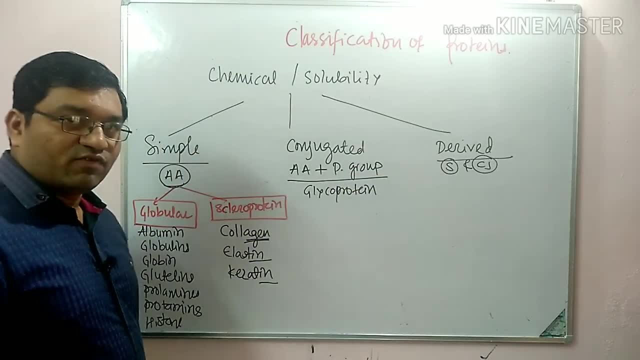 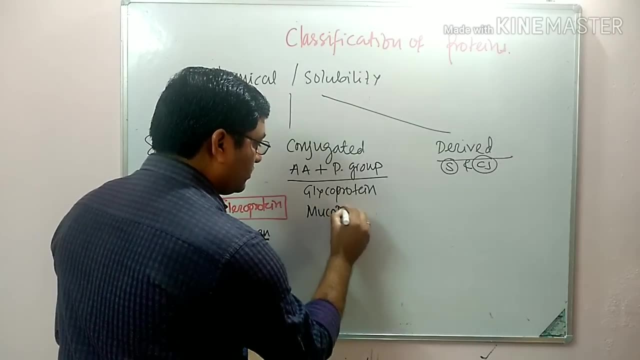 When content is less than 4%, it is known as Carbohydrate. When content is less than 4%, it is known as Glycoprotein. When it is more, it is known as Mucoprotein- Mucoprotein. 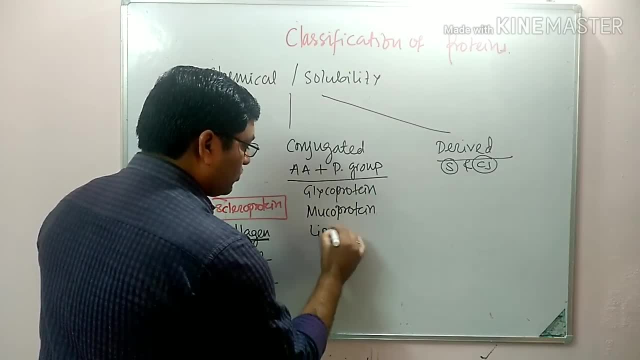 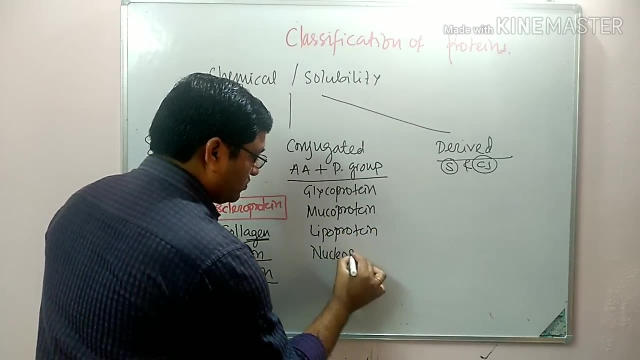 Okay. When it is associated with Liquid, it is known as Lipoprotein. When it is associated with Nucleic Acid, it is known as Nucleoprotein. When prosthetic group it is a colored substance, it is known as Chromoproteins. When there is metal incorporated in it as a prosthetic group, it is known as Metalloproteins. So this is a classification of Conjugated Protein: Glycoprotein, Mucoprotein, Lipoproteins, Nucleoproteins, Chromoproteins, Metalloproteins. 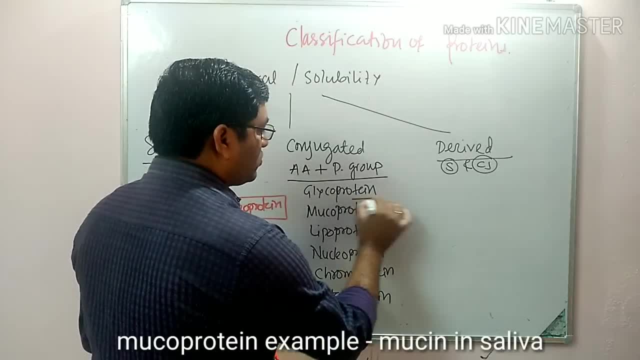 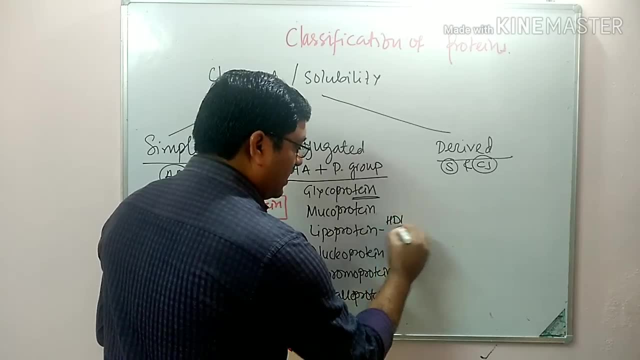 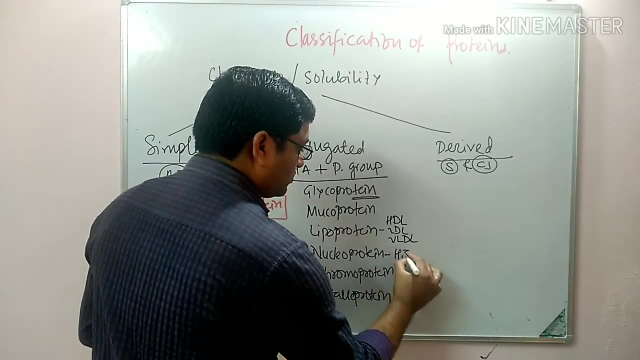 Okay, Blood group antigens. they belong to Glycoproteins. Okay Then Lipoproteins. you know the Lipoproteins: HDL, LDL, VLDL, etc. Nucleoproteins, Histones and Protamines. 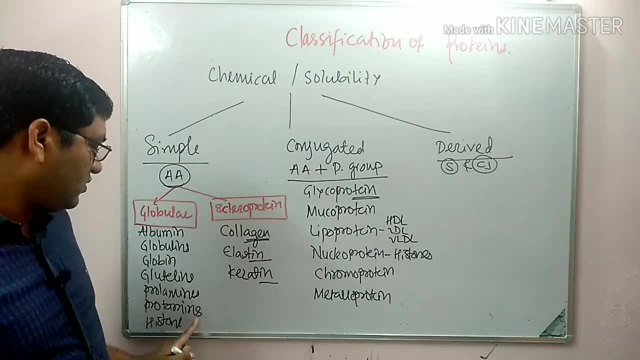 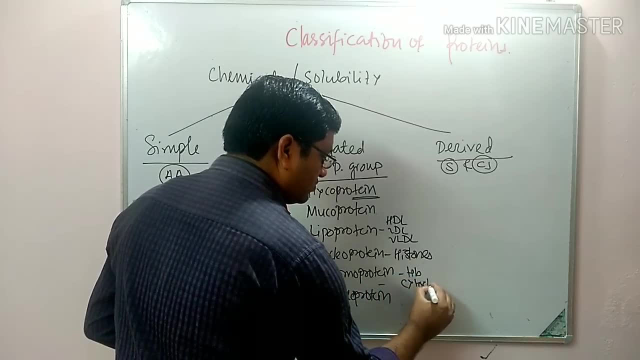 Protamines- they are found in the Histones And Nucleoprotamines. Okay, Then Chromoproteins, Hemoglobin, Then Cytochromes. They are Chromoproteins, Metalloproteins. most of the enzymes they contain metal. 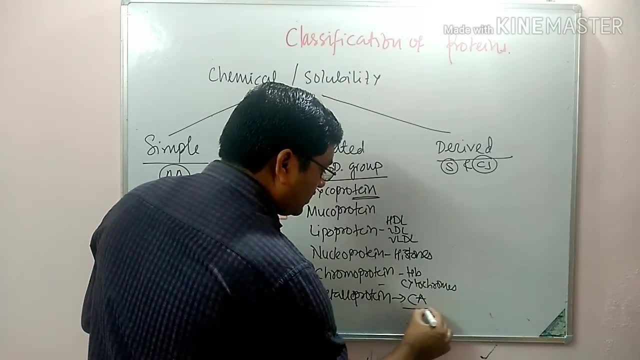 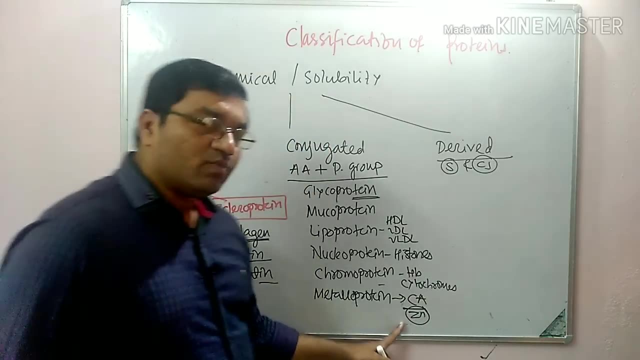 For example, Carbonic Anhydrase. Carbonic Anhydrase: It contains Zinc. Zinc is a metal. It is found in more than 300 of enzymes, Maximum in Dehydrogenase RNA Polymerase. Carbonic Anhydrase. 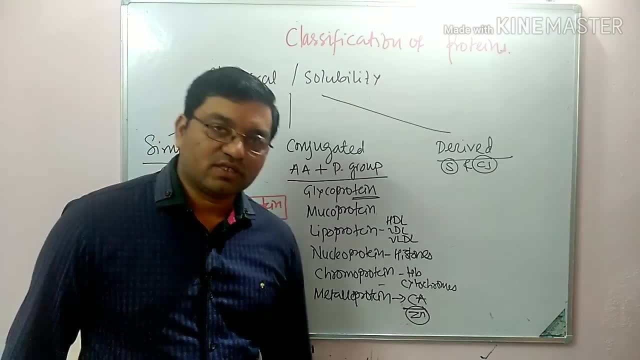 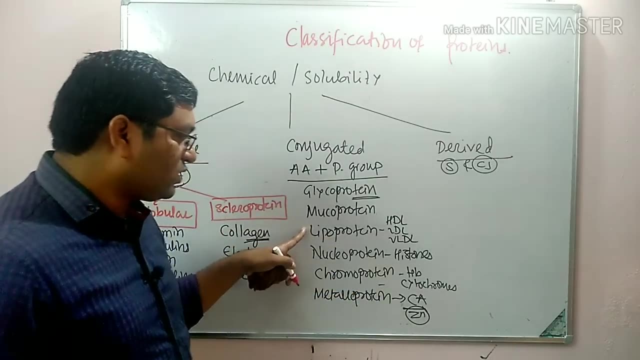 Superoxide Dismutase. Zinc is there? Okay, So Metalloprotein? So these are the examples: Glycoprotein, Mucoprotein, Lipoproteins, Then Nucleoproteins, Chromoproteins, Metalloproteins. These are the examples: Glycoprotein, Blood group antigen, Then Lycoproteins, HDL, LDL, VLDL, Histones, Nucleoprotein, Hemoglobin, Cytochrome, Chromoprotein and Metalloprotein. 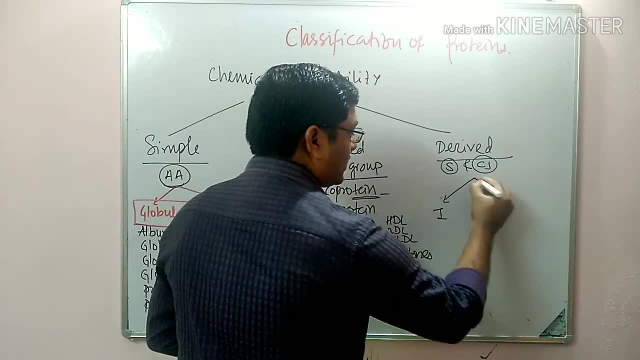 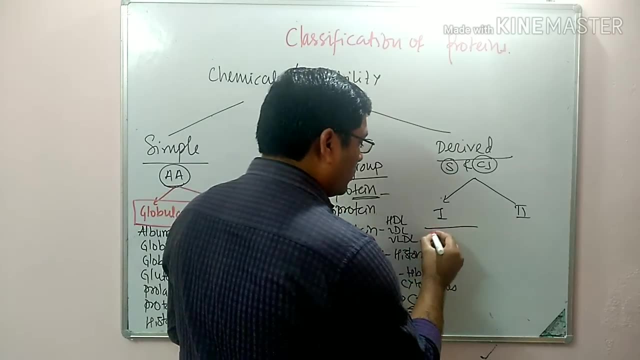 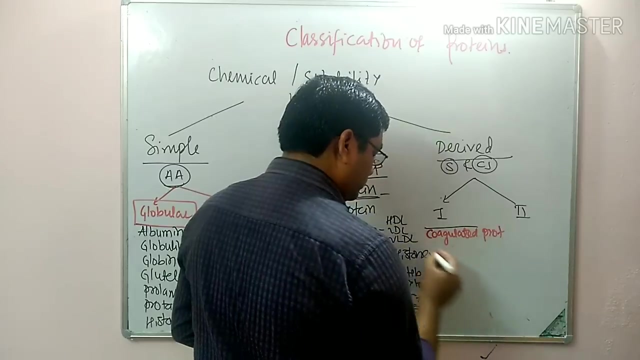 Then Derived Protein. it includes primary Derived Proteins And Secondary Derived Proteins. Okay, These primary includes Denatured and Coagulated Proteins, Coagulated Proteins, Denatured and Coagulated Proteins, Then Proteins. 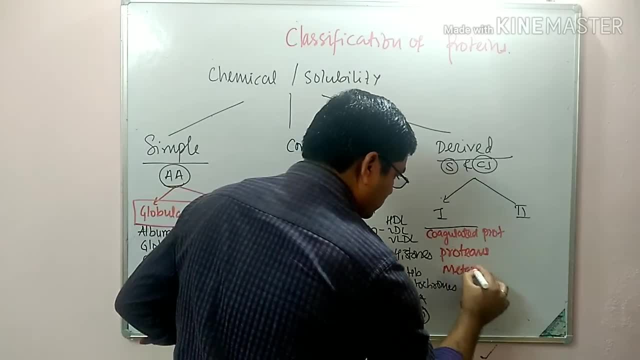 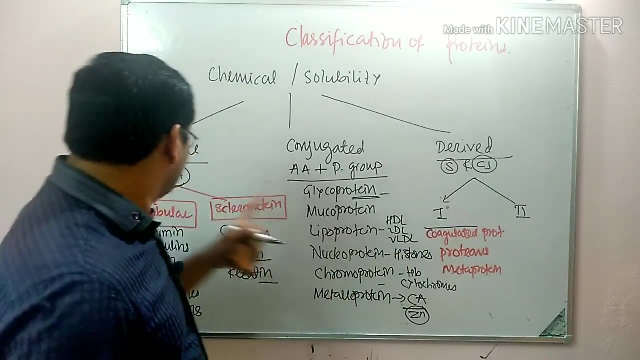 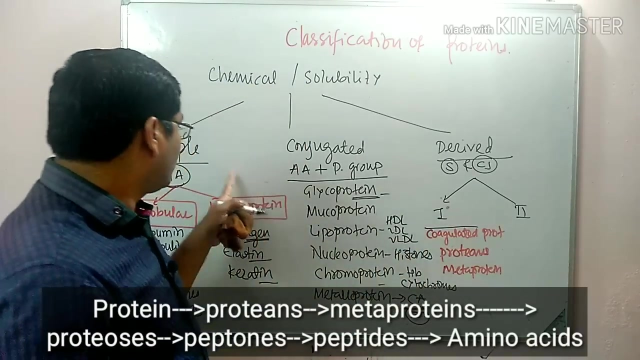 And Metaproteins. Metaproteins: These primary Proteins. They are primary hydrolyzed product of these simple and conjugated protein. Primary hydrolyzed product. They are coagulated or denatured product of simple and conjugated protein. 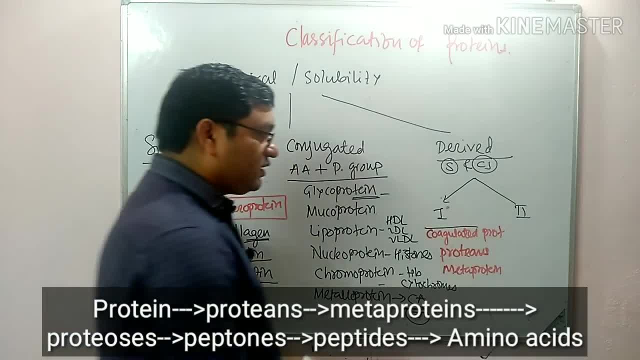 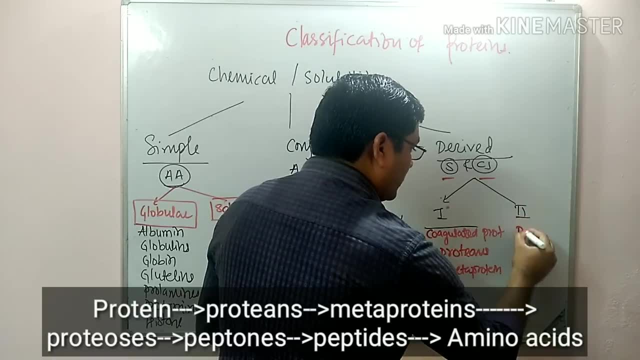 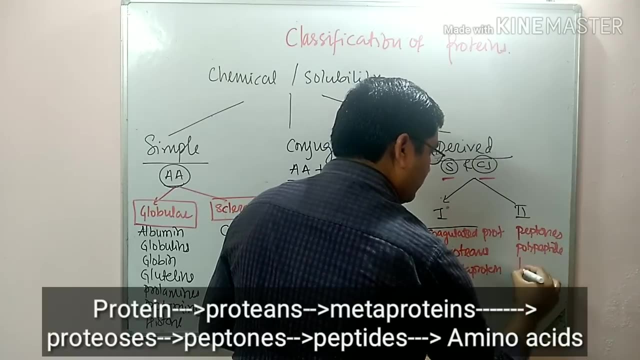 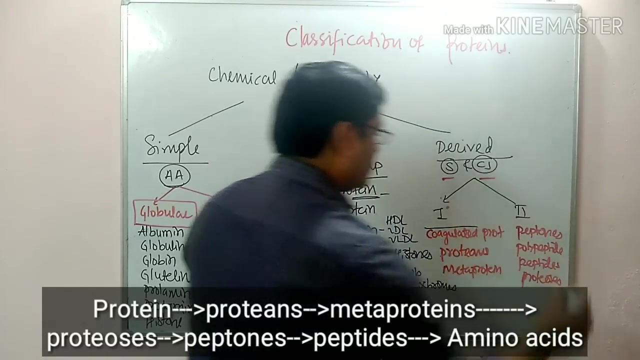 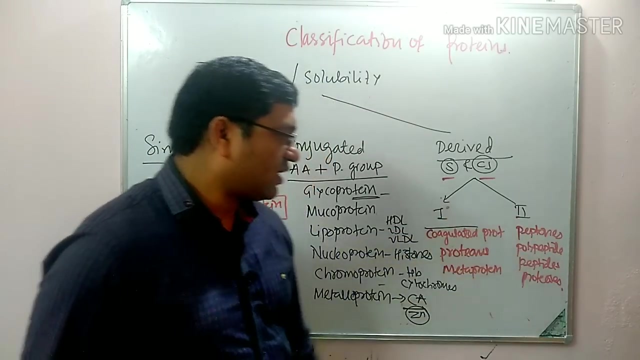 They belong to primary And secondary. they are: on further hydrolysis of simple and conjugated protein, We get secondary proteins, Which includes Peptones, Polypeptides. So they are included in the secondary Derived Protein: Peptones, Proteases, Polypeptides and Peptides. 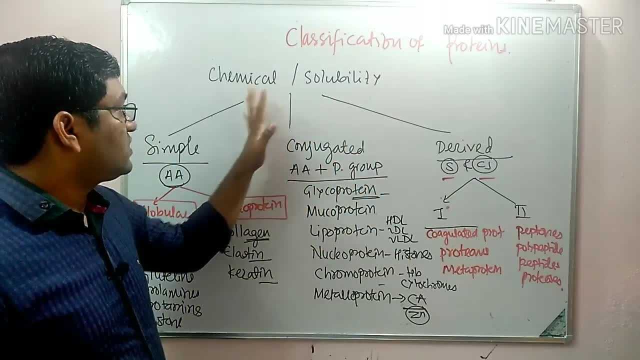 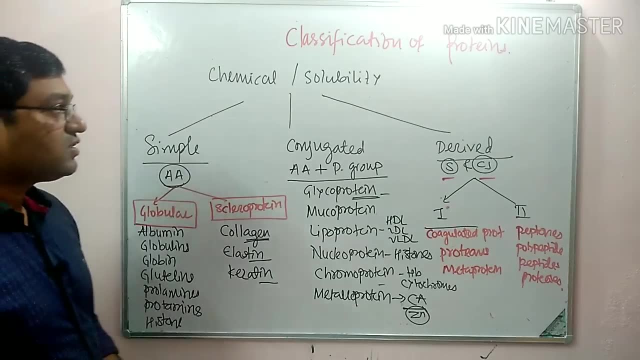 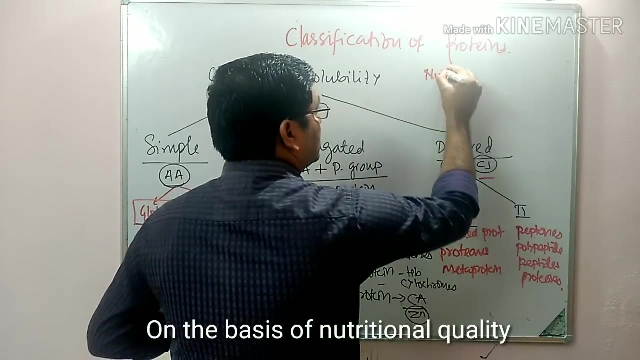 Okay, So this is all about the classification of protein based on their chemical nature and solubility. Take a snapshot here. Okay, Now we will discuss about: Okay, The Nutritional Classification. In Nutritional Classification, Nutritional, there are three groups. 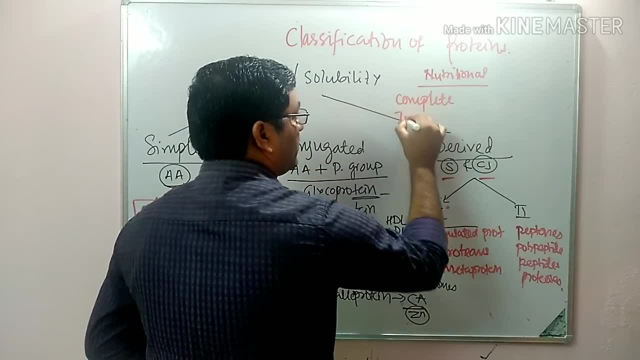 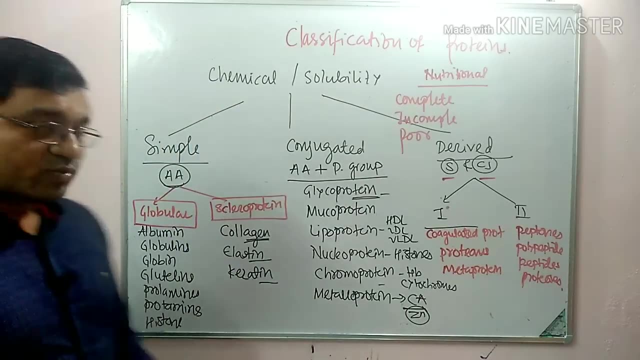 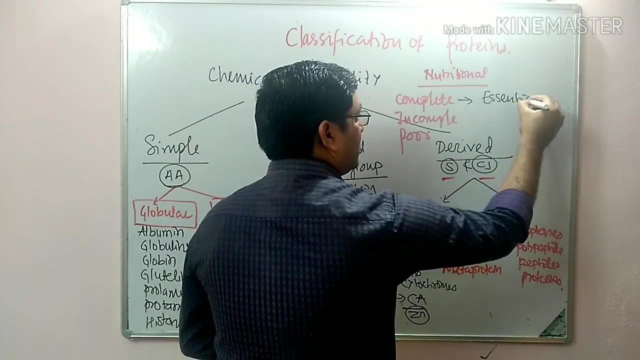 Complete Protein. Complete, Incomplete and Poor Protein. Complete, Incomplete and Poor Protein. Those Protein which contain all Essential Amino Acids. Essential Amino Acids- Essential- means you know the mnemonic that Matt will fly. 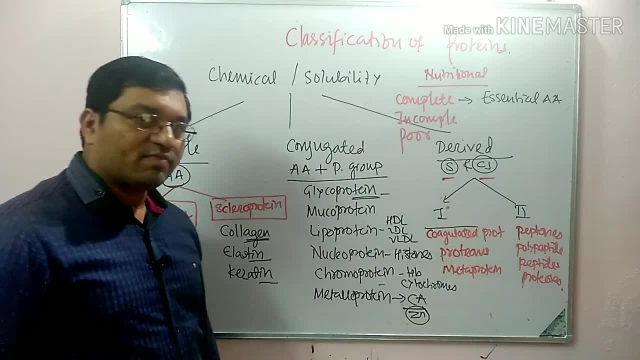 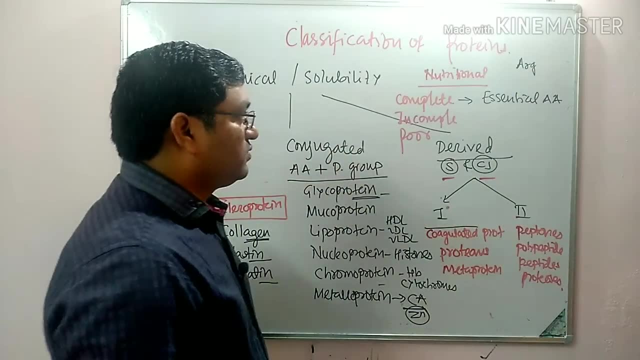 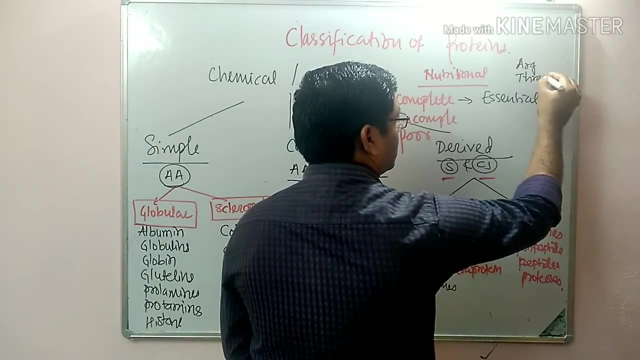 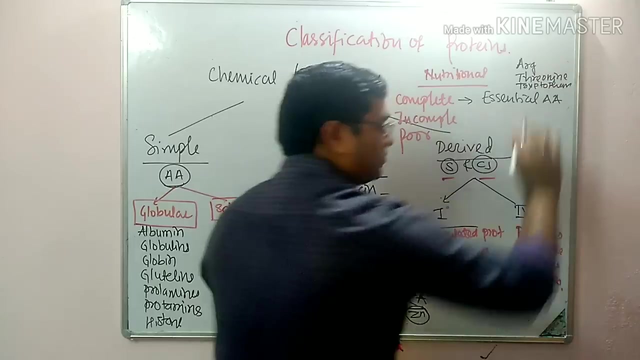 That is for Essential Amino Acids In Matt will fly. remember. A for Arginine- is there Arginine? is there, Okay? And T for Threonine and Tryptophan- Okay, There is no Tyrosine in Essential Amino Acid because Tyrosine is synthesized from Phenylalanine. 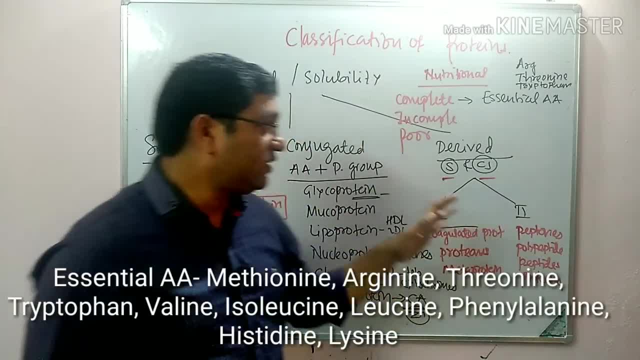 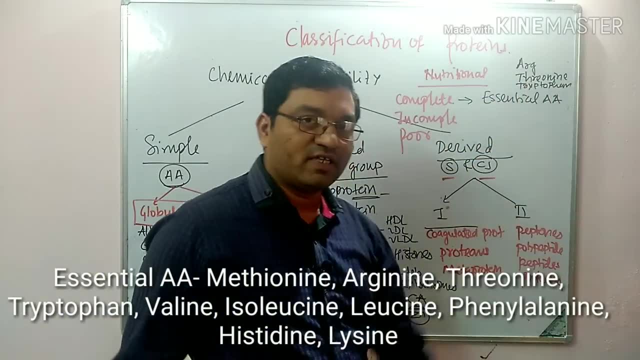 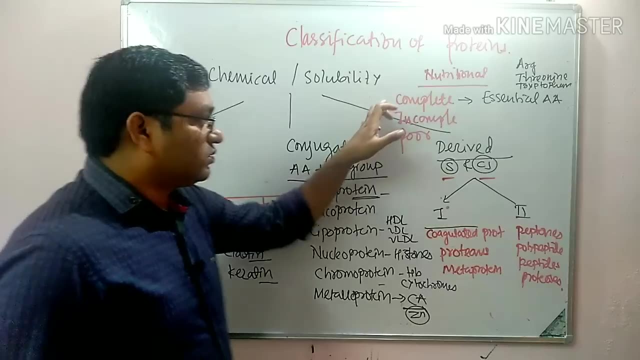 So in Matt will fly M-A-T-T-V-I-L-P-H-L-Y, So A for Arginine, Threonine and Tryptophan is there No Tyrosine, So Matt will fly. Complete Protein containing all Essential Amino Acids. 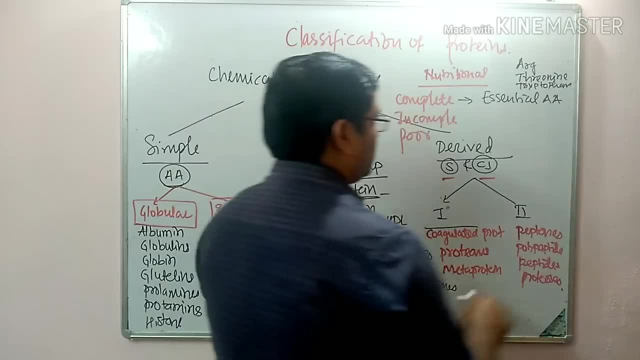 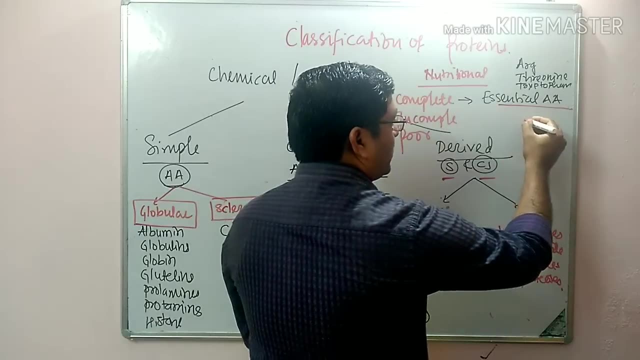 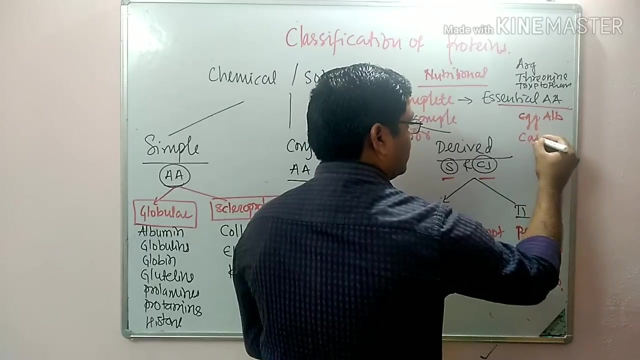 They are known as Complete Protein Example, as per body requirement Means they contain all Amino Acids as per body requirement. They are known as Complete Protein Example: Egg Albumin, Egg Albumin and Milk Casein. Milk Casein also belongs to Phosphoprotein.